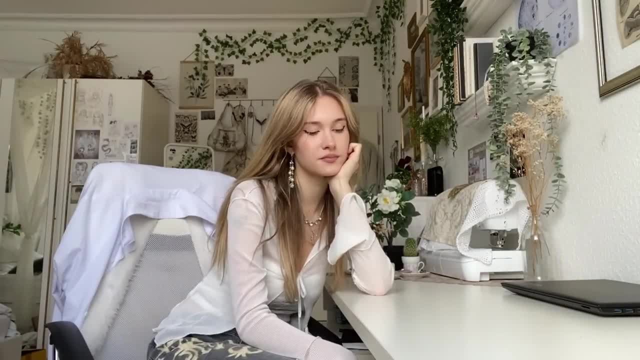 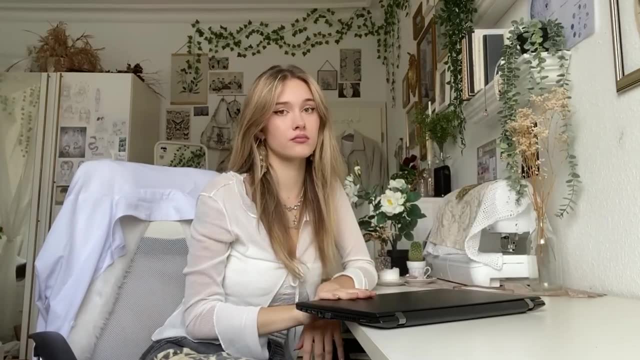 I think we all had the problem before of not knowing a present to give to our friend, family or a loved one, Like there are so many options and you just kind of feel overwhelmed. So today I want to show you some DIY gifts you can make with stuff you might have already at home. 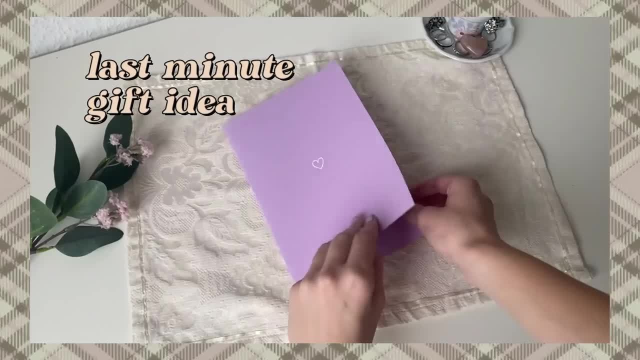 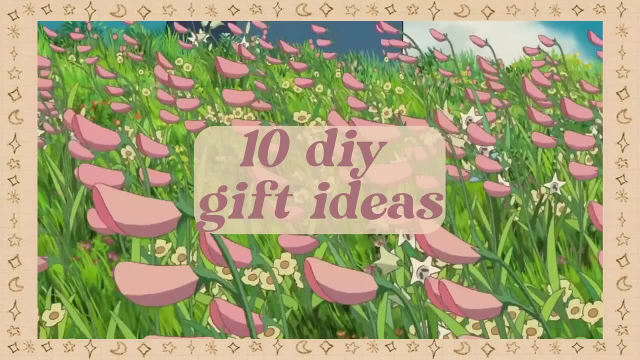 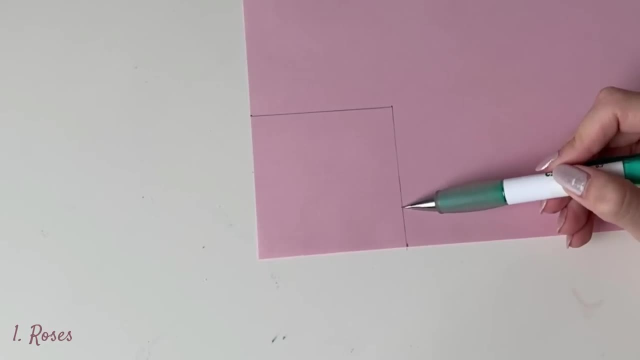 They are so easy to make and look super aesthetic. So if you need any last minute gift idea or you're just looking for cute DIY gifts in general, watch this video: 1000 höhenzüge. So first we have these tiny but super pretty roses. You just have to fold the paper on one side. 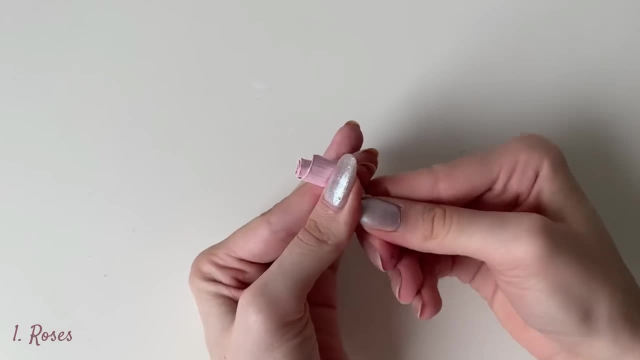 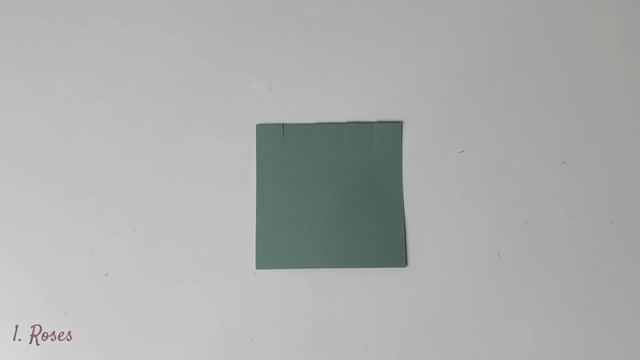 then roll it and twist the bottom so it creates this rose shape on the top. Grab a second piece of paper and cut some slits in it To make it look like leaves. fold the sides on each slit so it looks like this. Then put the first paper in it. 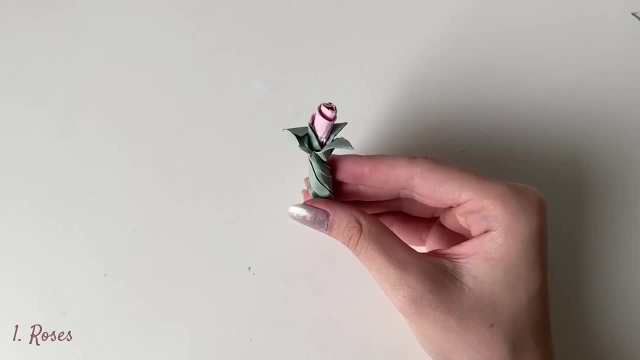 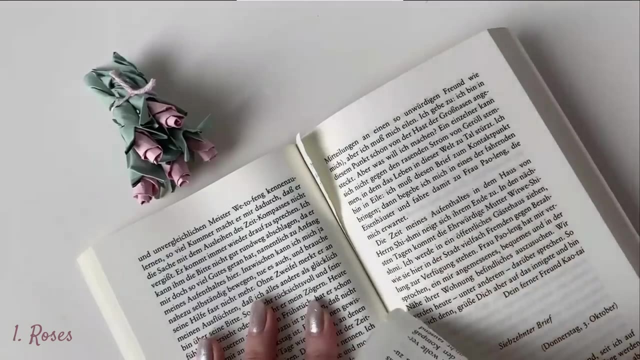 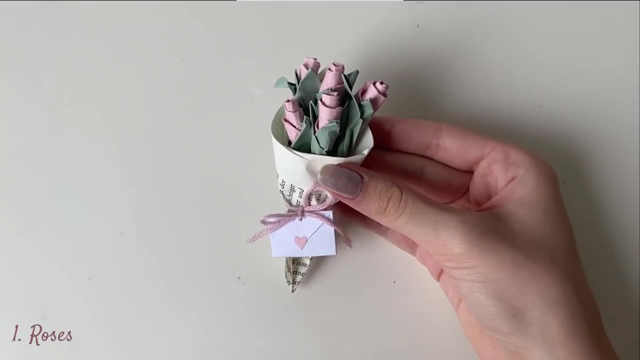 And roll everything once again. So now you have this really pretty rose, Repeat it a bunch of times and tie them together. I put a piece of paper from a book around it to make it look a little more aesthetic and added a tiny letter, And this is how it turned out in the end. 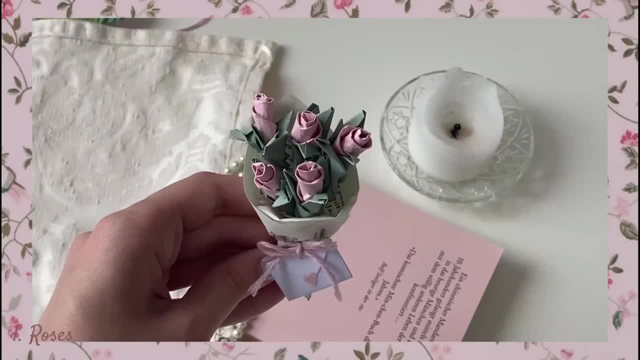 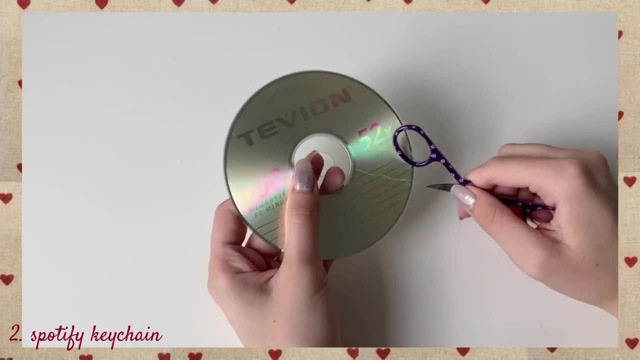 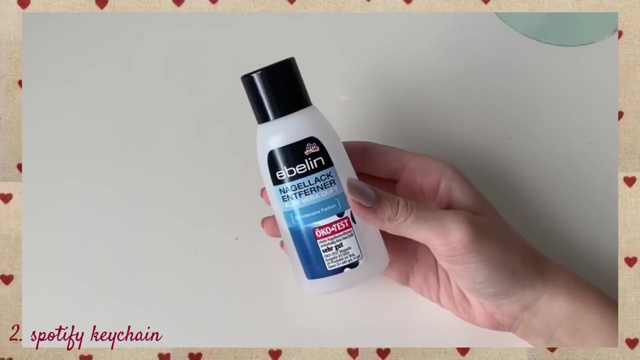 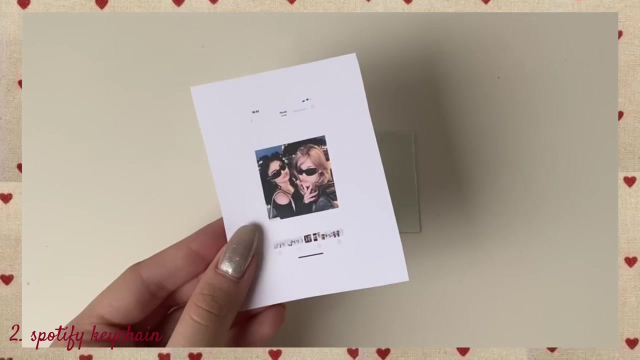 Now I'm showing you how to make a Spotify keychain. First, remove the shiny part of a CD by pulling it off with some tape and rubbing some nail polish remover on it to get rid of the greenish tint. Next, you're gonna cut out two squares and print out a pic of your choice, but you can also draw. 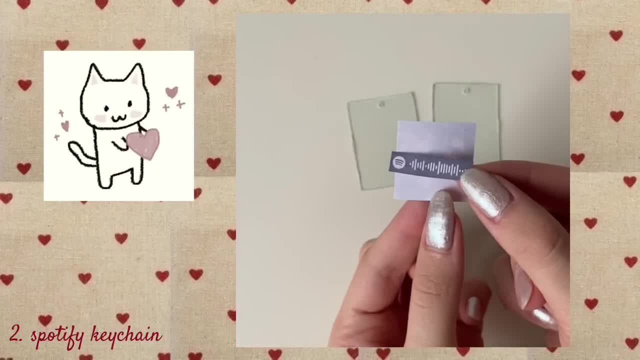 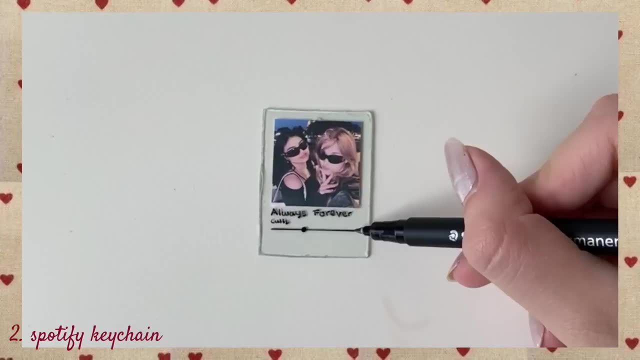 a cute image like these ones I found on Pinterest. I added a Spotify code of songs that remind me of my friend on the back and glued it on the CD Beneath it. I drew some things to make it look like a song on Spotify and glued the second CD on top. 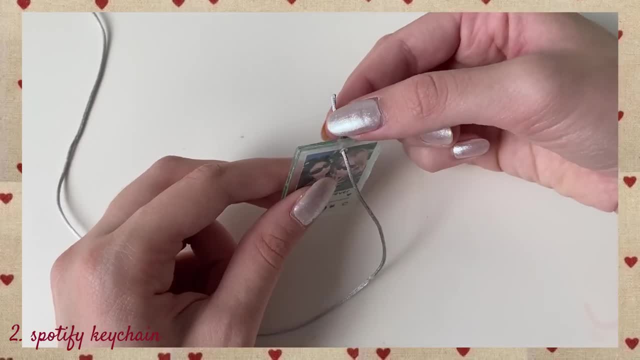 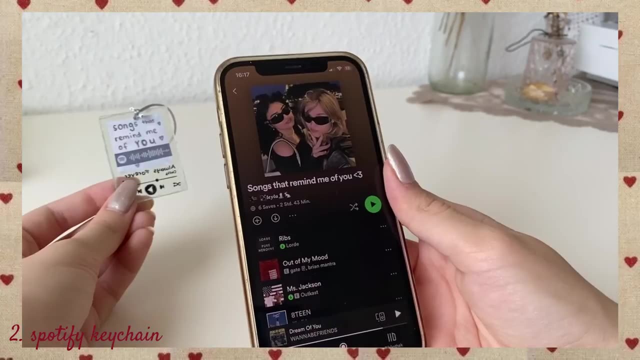 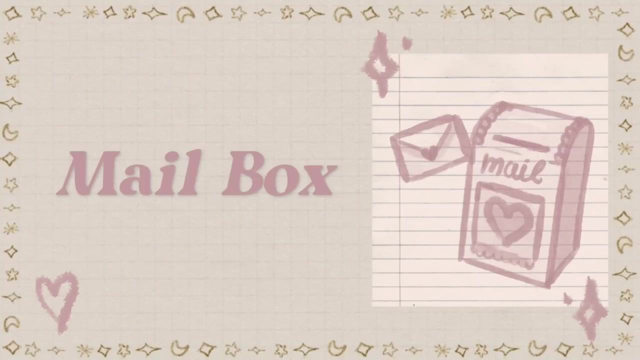 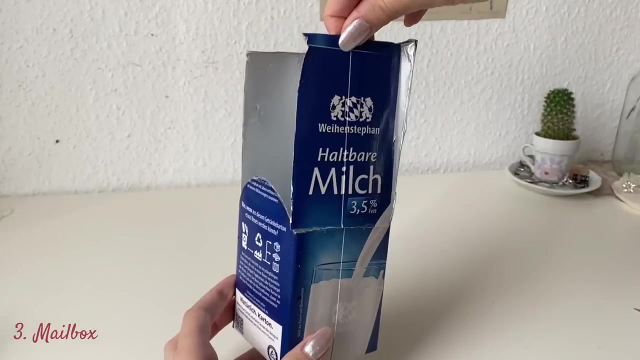 Now all there is left to do is to add a string and you're done. This way, your friend has a cute keychain where they can listen to your playlist any time of the day. If you want to share a message in a cute way, this DIY is perfect for you. Just cut a curve in the 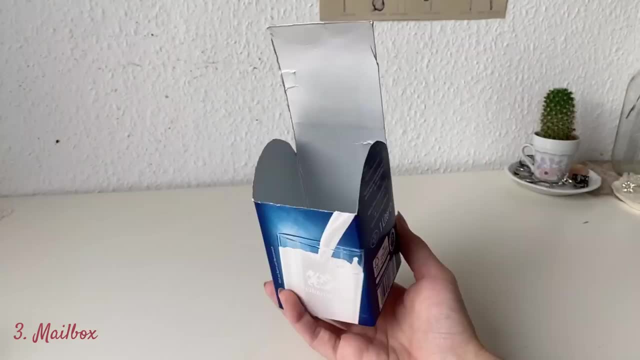 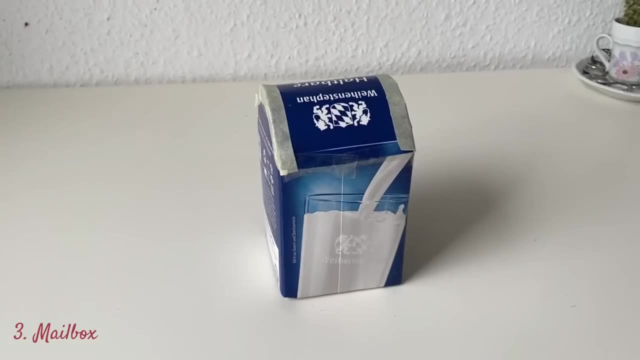 middle of a milk packaging and remove the sides so it looks like this. Then use some tape to create this box shape and put some more down on each side to close up the open edges, After cutting a small slit and a square beneath it. cover everything in paint and add some decorations. 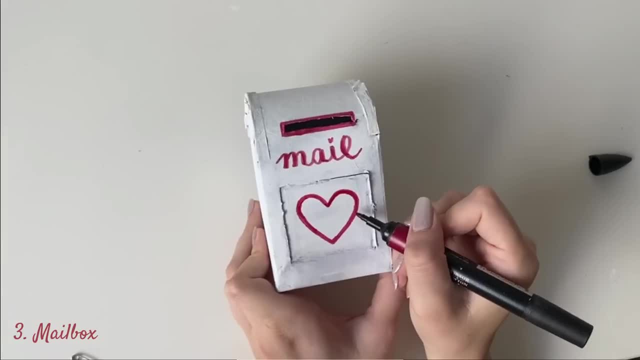 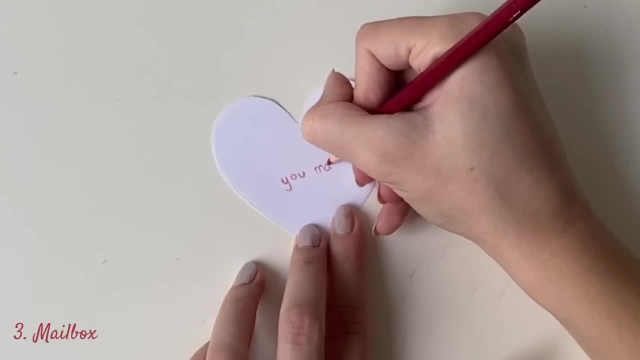 with a marker. I think a mailbox is a very creative way to decorate your home, To write letters about all sorts of things to your friend. You can write down things you like about your friend, an activity you can try out together or just a message you want to share. 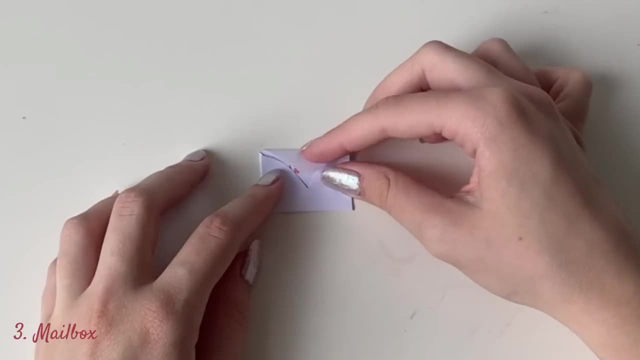 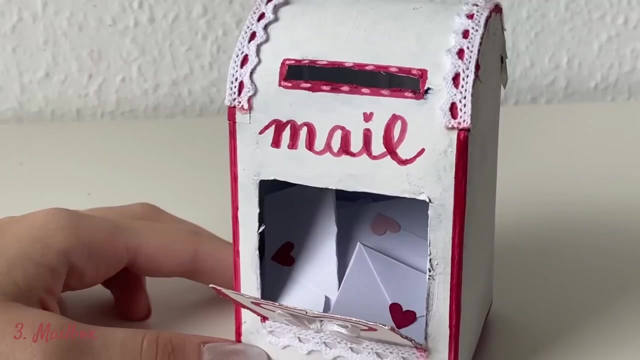 I made some letters in a heart shape. then I folded the paper and glued a heart on it to keep everything in place. I made a bunch of these and filled a mailbox with them. So now, when your friend feels like it, they can enjoy your tiny love letters. 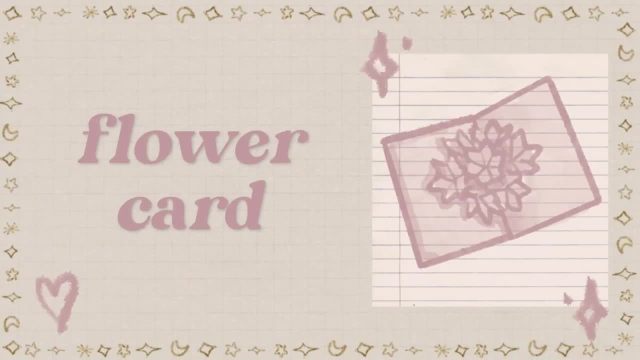 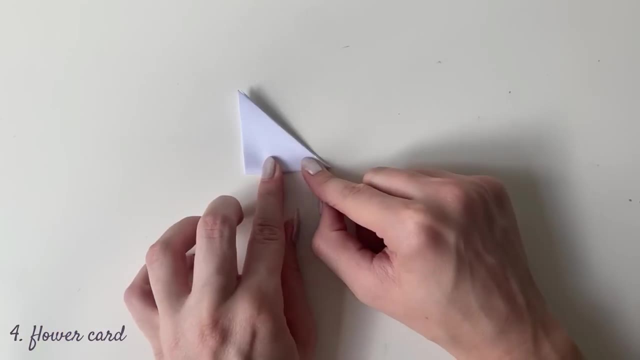 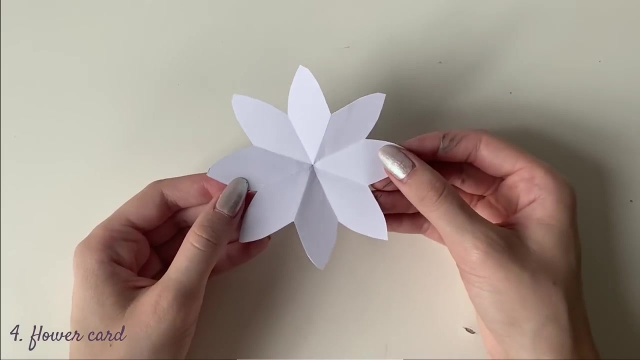 I think everyone has gotten a card for their birthday at some point, but I want to show you how you can make a card that your friend has never seen before and looks so aesthetic. You just need to make a bunch of origami flowers. I chose a purple pencil to add more color to. 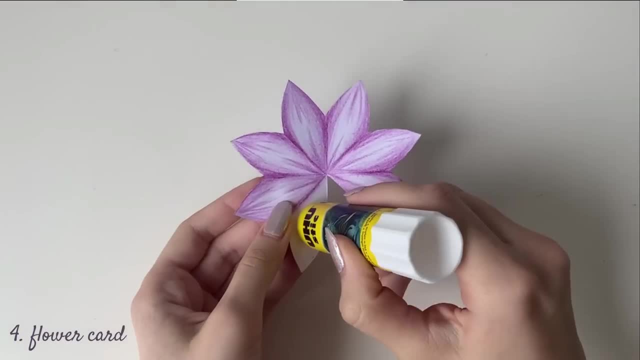 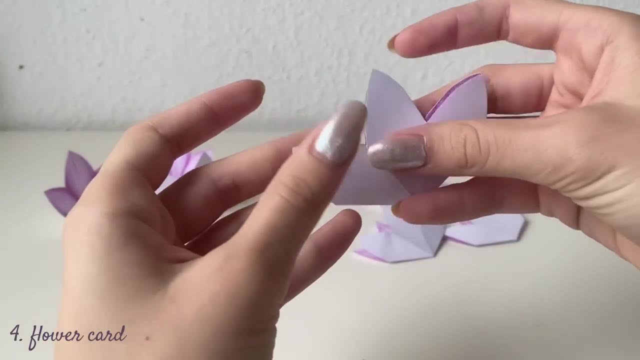 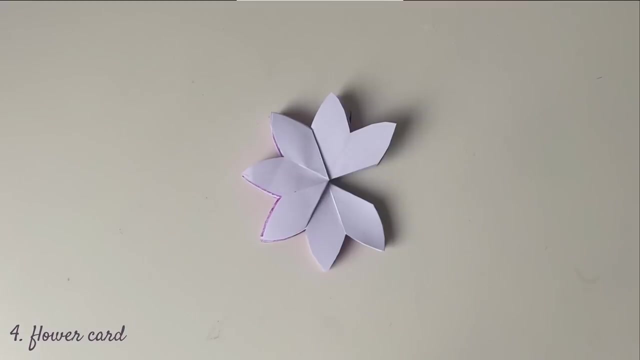 the flower and then I cut out one part and glued the other one on top to make it look 3D. I repeated 10 times until I had a bunch of cute flowers. Now put some glue on specific ends of the flower. It's very important where you put down the glue, so make sure you get this part correct. 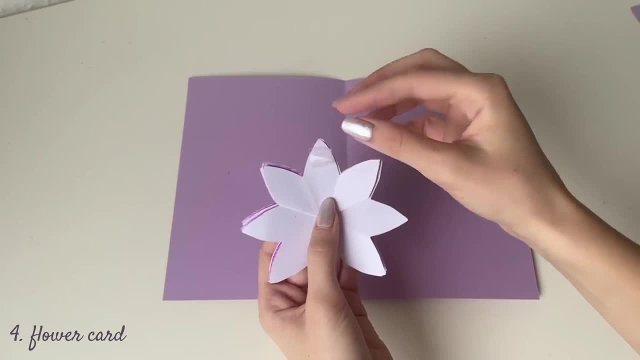 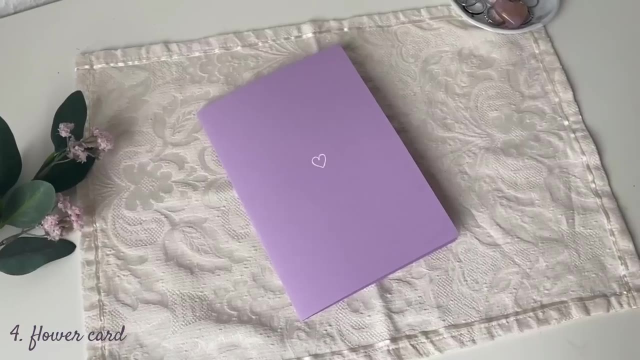 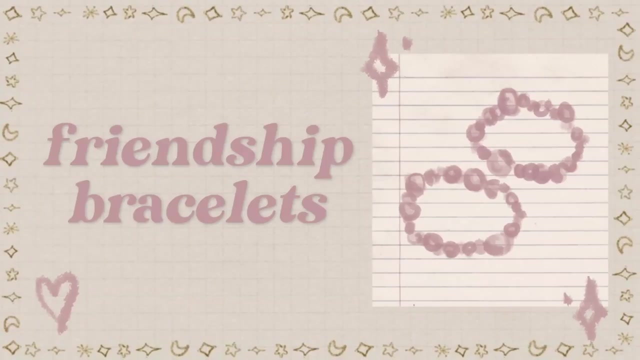 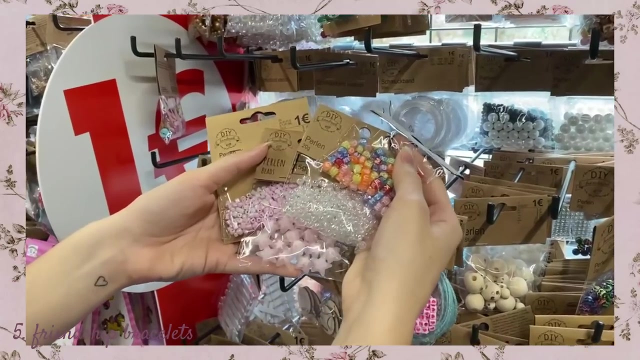 When you're done, it should look something like this: Put a piece of tape on both ends and lay it in a folded paper, And that's how you get this gorgeous 3D flower card. For this DIY, I just went to a dollar store and picked a bunch of pearls. 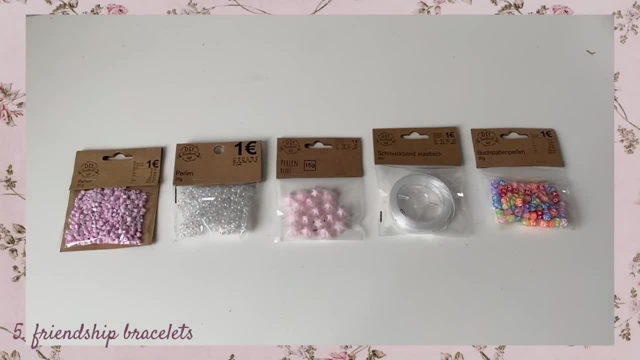 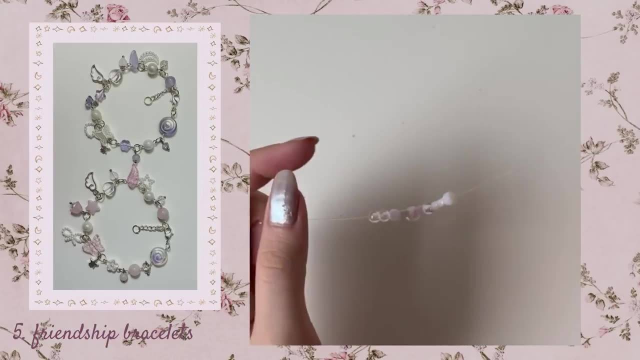 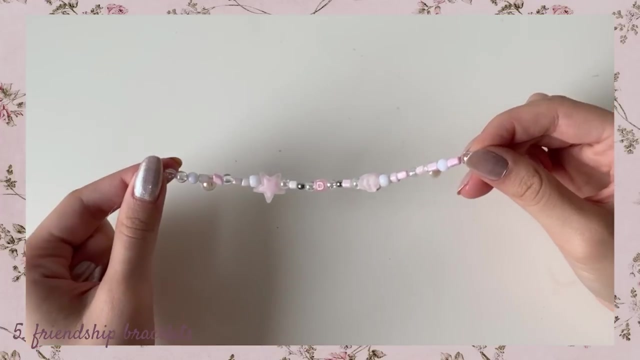 I got some in the colors pink and white and also some letters. If you want some inspo of pretty friendship bracelet designs, I recommend looking on Pinterest so you can try to recreate them. I just switched between each pearl and in the middle I added the initial of my friend to make it more personalized. so it turned out like this: 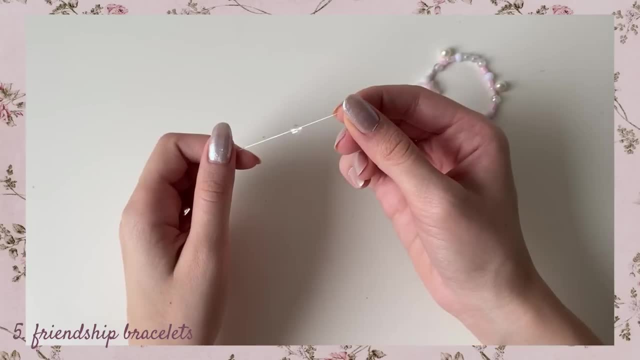 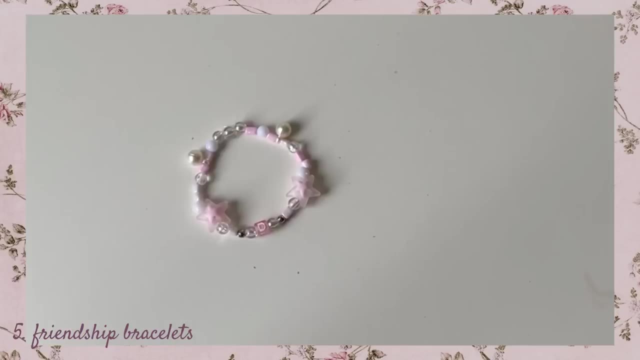 When you're done, tie a knot and repeat the process a second time, but add your initial instead. I think friendship bracelets are so cute because they not only look very aesthetic, but you also carry around something that reminds you of your friend no matter where you are, which makes this the perfect gift. 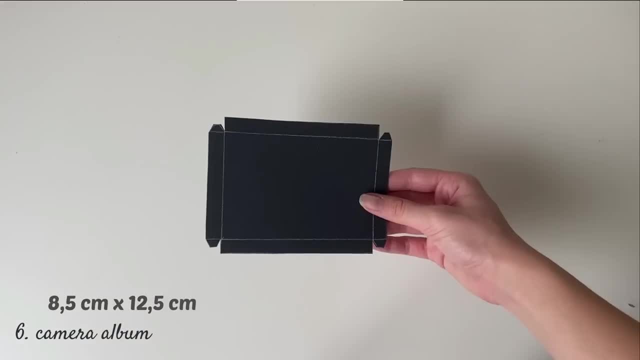 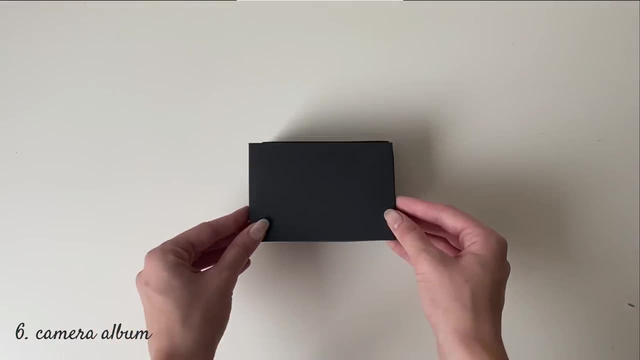 If you want to make a gift where you can look back at all the fun memories you've experienced with your friend, you should definitely try out this DIY Here. I recreated a photo camera by using some black paper to create a box. I drew a few things to decorate the camera like this. 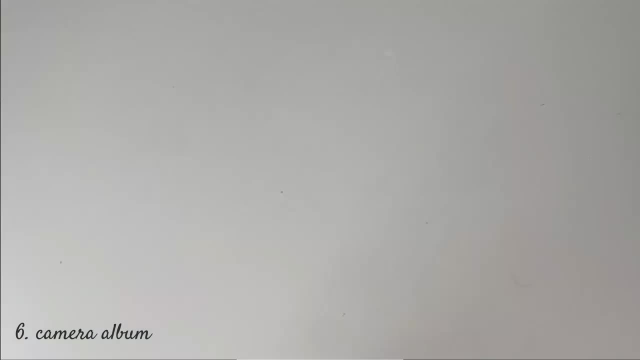 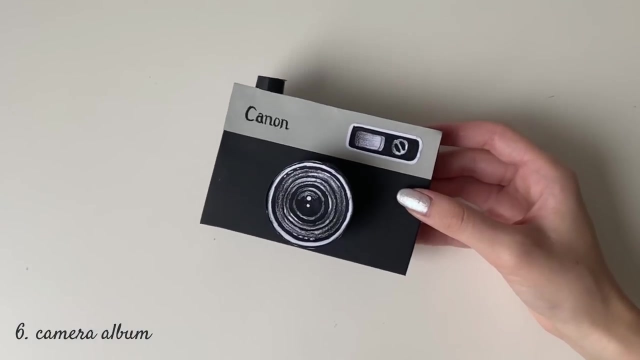 lens. here I added this black piece of paper to make it look 3D, and with everything ready, I got to adding all the details. I think a camera is the perfect thing to use for an album, because it looks like it captured all the fun things that you did together. So 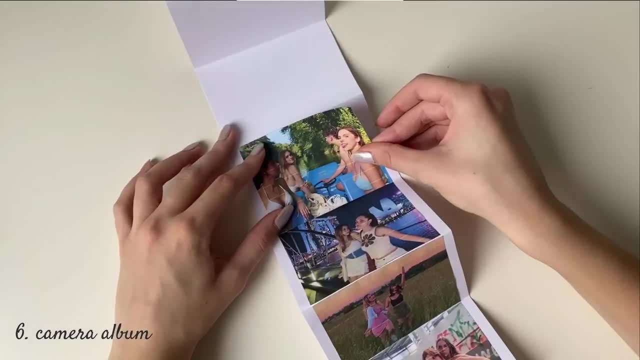 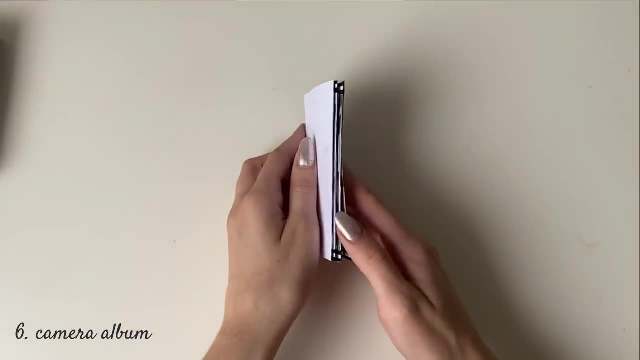 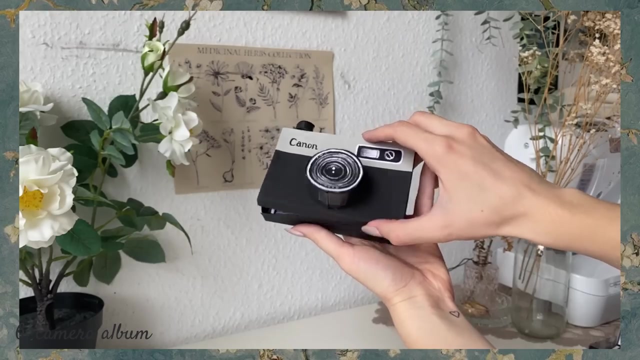 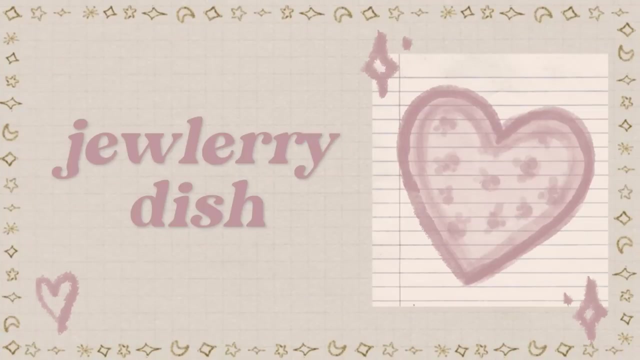 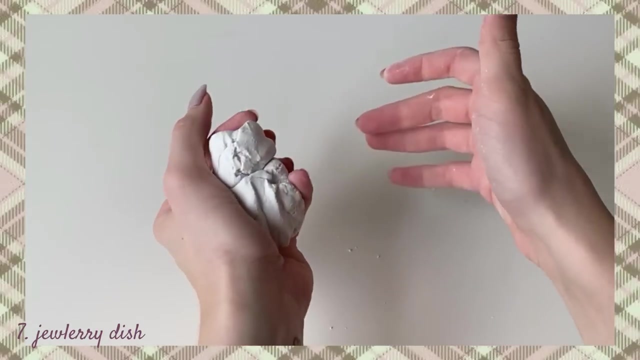 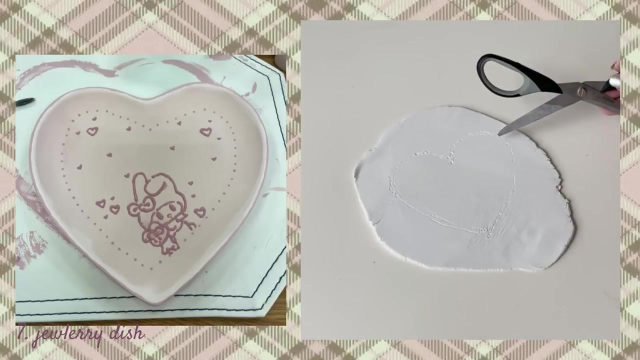 print out your favorite pics and glue them on the fold, And here you have your finished Bible camera. Jewelry dishes are not only super pretty and aesthetic, they are also very useful And very fun. of course, friend is a person who owns a lot of jewelry. this gift is perfect for them. there are also many cute. 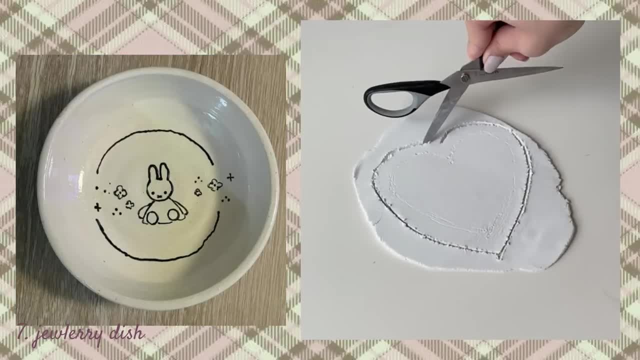 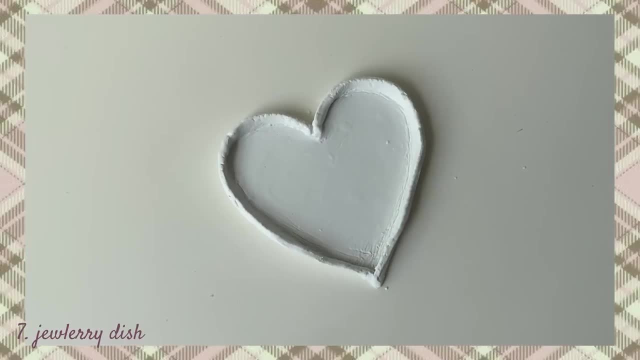 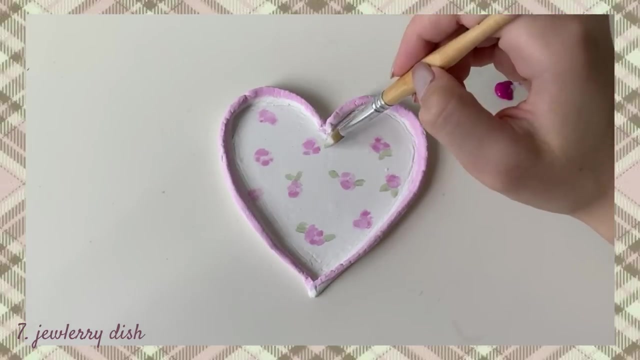 jewelry dish designs you can try out, so here are a few i found on pinterest. i decided to make one in a heart shape, so i just formed a heart into the clay like this. now paint a dish however you like. i painted some small roses on there and also added some leaves. this is how it turned out in the end. 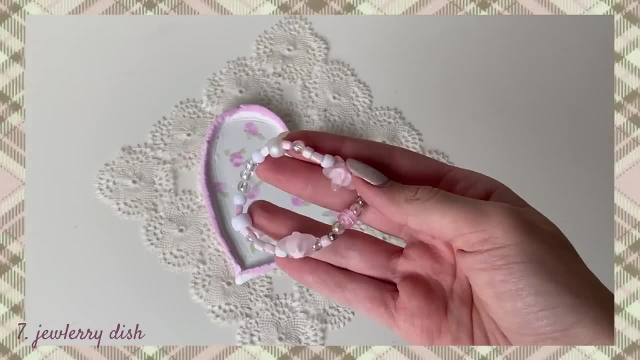 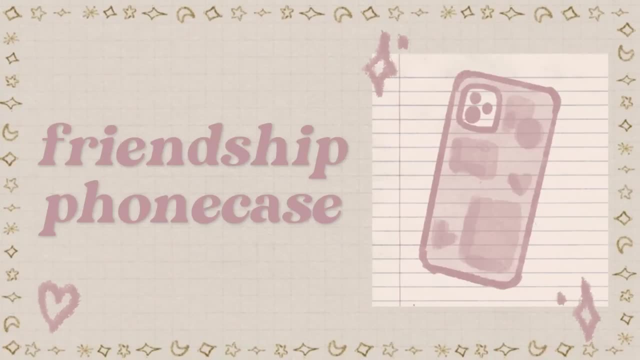 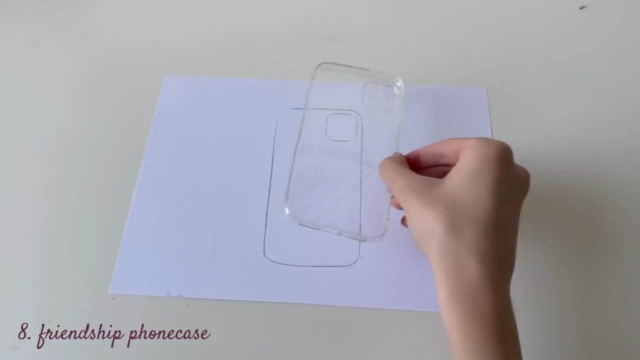 and i think it looks so cute. and, by the way, the perfect thing to go with this gift is a diy friendship bracelet. you can also make a custom phone case for your friend. here i outlined the shape of a clear phone case and cut it out. then i decorated the piece with some images i printed out. 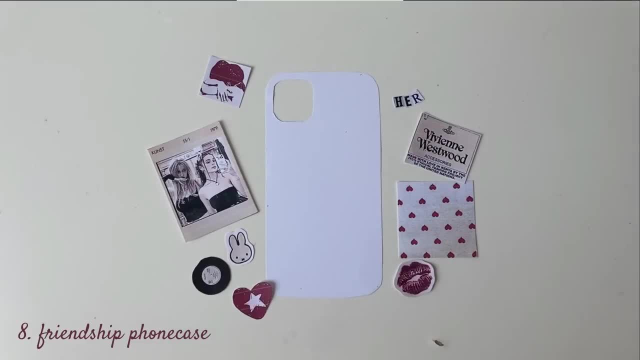 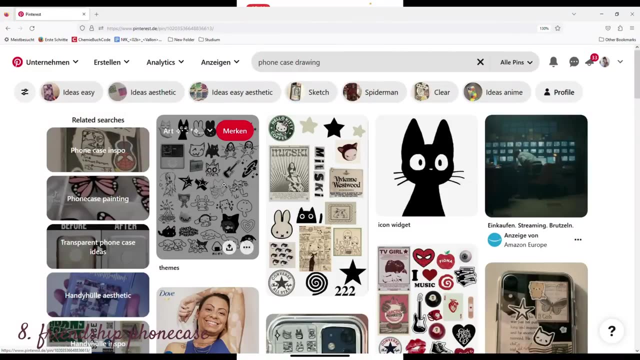 i found these on pinterest, so i really recommend looking there if you want some inspo, because there are so many in the shop. see you next time, many cute phone cases like these ones. and, by the way, if you don't have a printer at home, 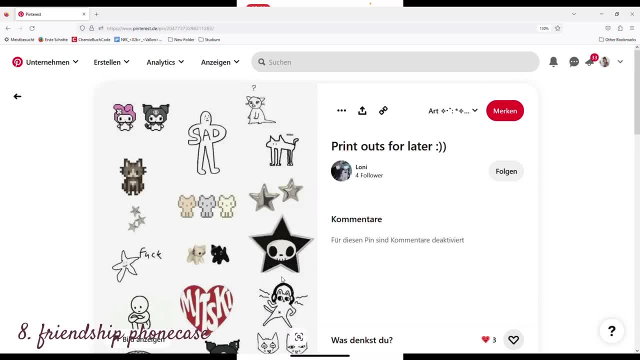 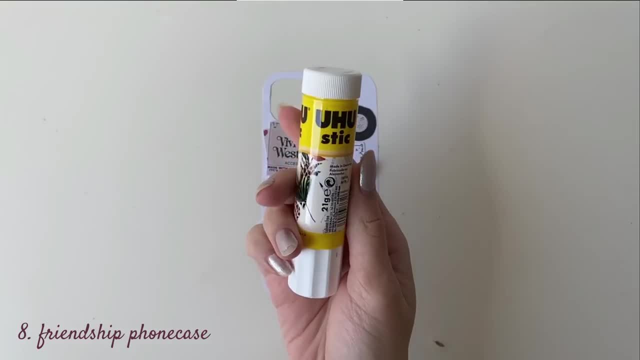 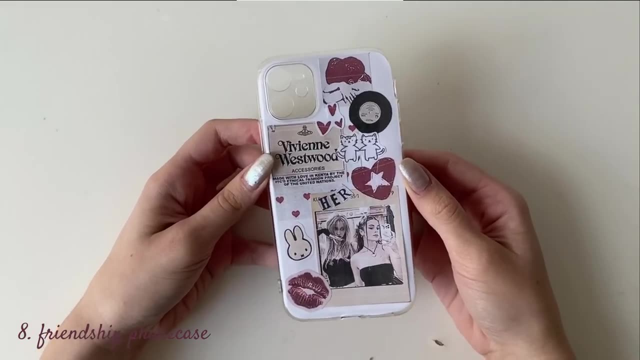 you can also draw a bunch of cute things like these images and glue them on your case. so first plan the layout till you found an arrangement that you like. then grab some glue and stick everything together, put the paper in the case and you're done. this is how my finished friendship phone case. 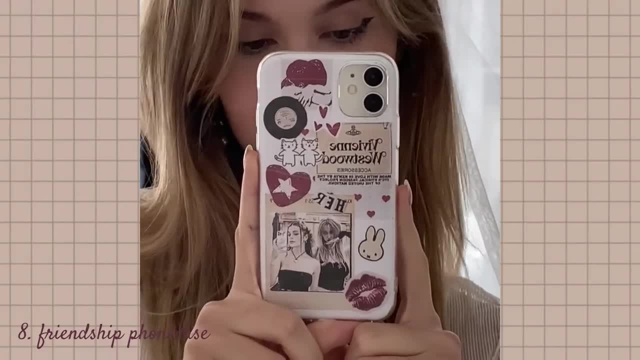 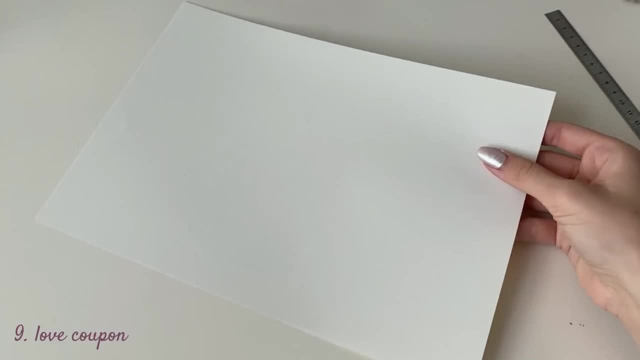 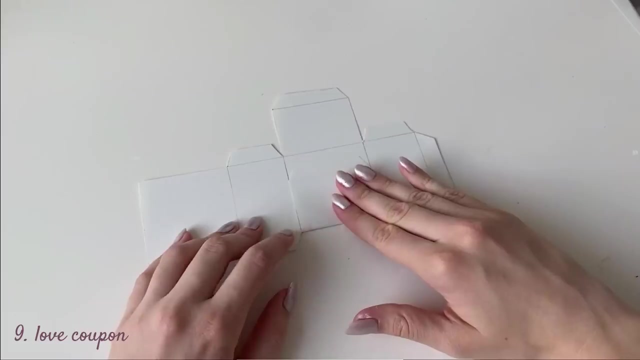 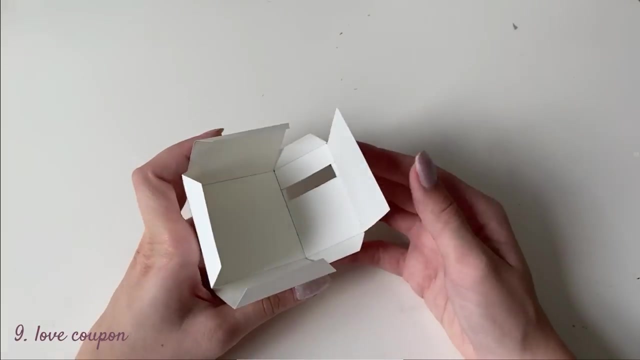 turned out. if you want to plan a bunch of cute activities you can do with your friend and put it in the form of a gift, this love coupon idea is perfect for you. i think gifting experiences instead of material gifts has sometimes a lot more benefits, because they 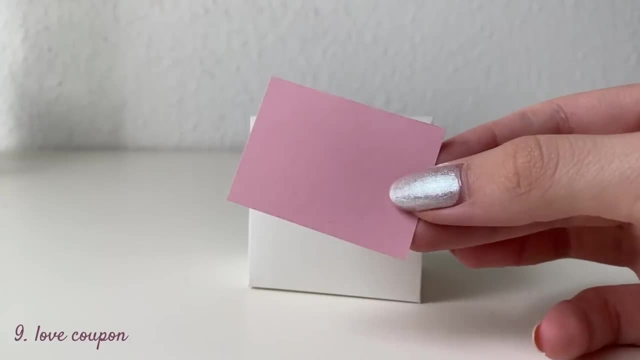 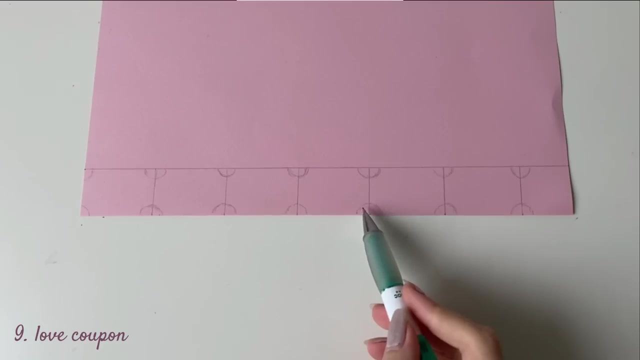 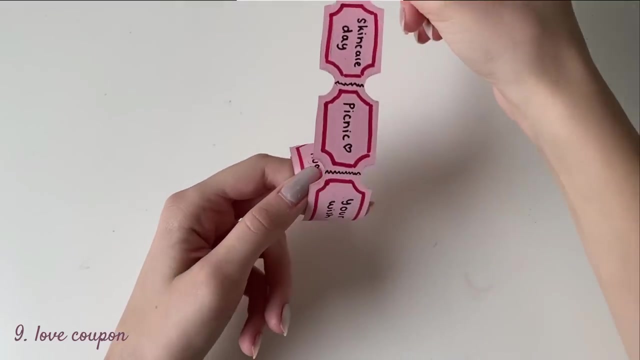 make unforgettable moments and you can just have fun together. so i made this tiny box with a slit and decorated it with some paper and a red marker. then i made some coupons and wrote cute things i want to do with my friend, like a movie night, a picnic or a skincare day. 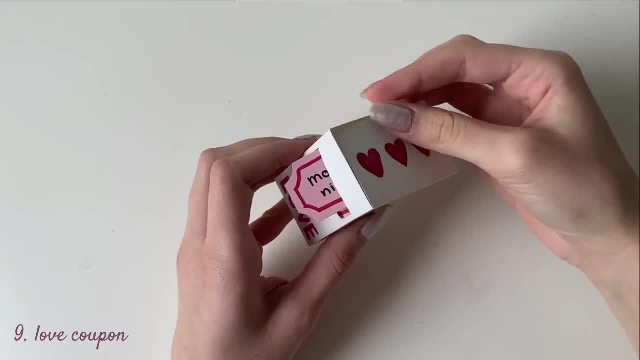 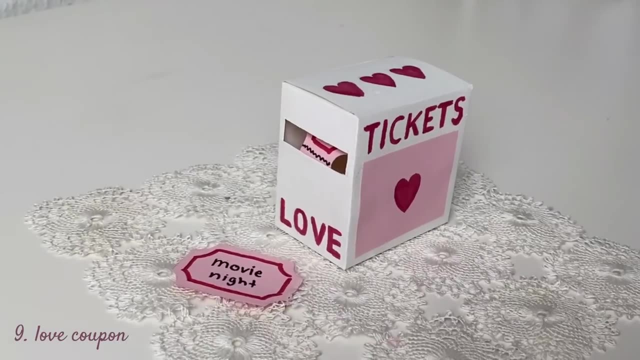 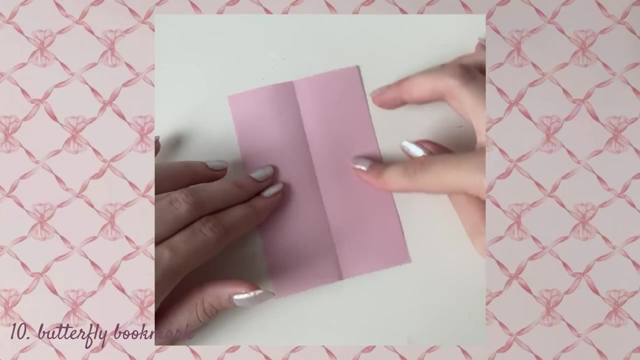 lastly, put the coupons in the box and you're done. now your friend can get a coupon whenever they want to and enjoy the cute activities you've planned. if your friend is a person who loves to read, you can also make a butterfly bookmark. all you need to do is to fold a piece of paper. 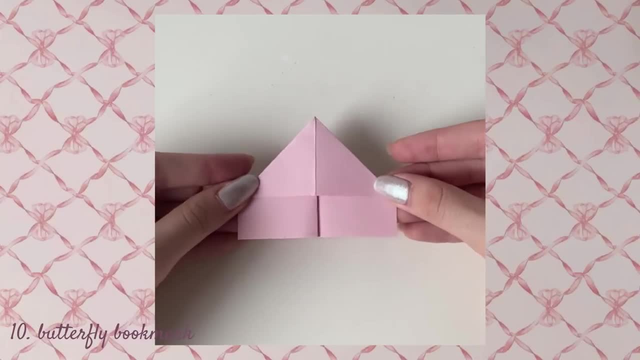 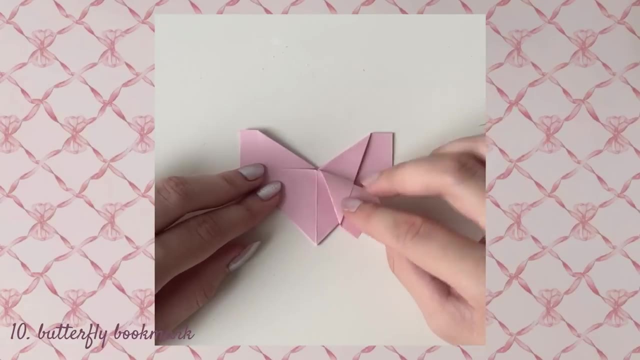 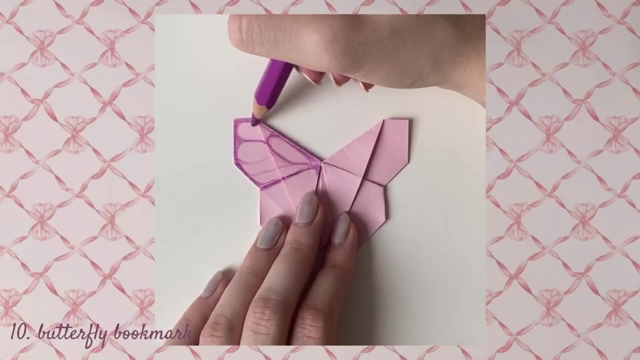 with the measurements 8 by 12 centimeters, like i did here. this diy is so easy to make and it looks so cute and aesthetic. after you've folded the last bit, it should look like this. you could stop here, but if you want to, you can also add a few details. i just added a few lines with a purple pencil and 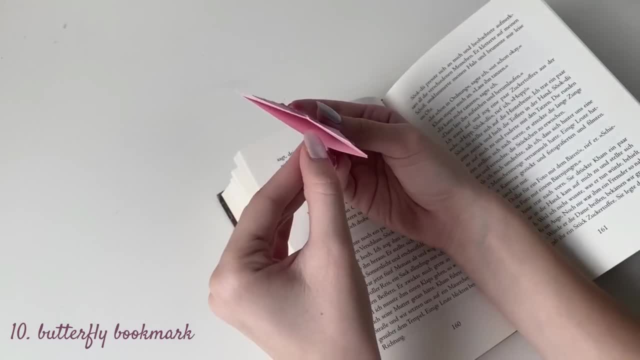 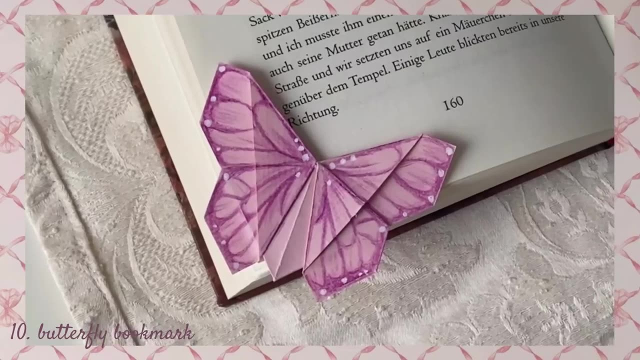 some dots. if you want to, you can also add a few details. i just added a few lines with a purple pencil and some dots. you can see there is a small open fold here, so if you want to use it, just put the page between it. and this is how our finished butterfly bookmark looks like. 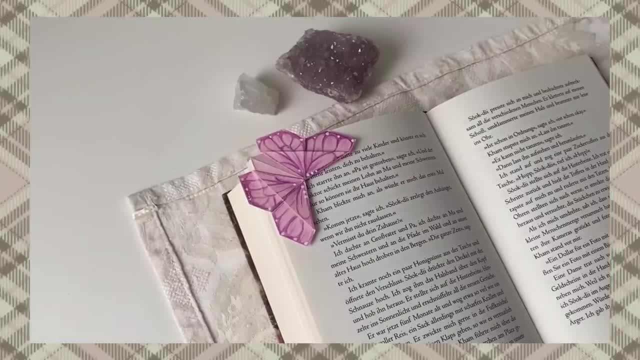 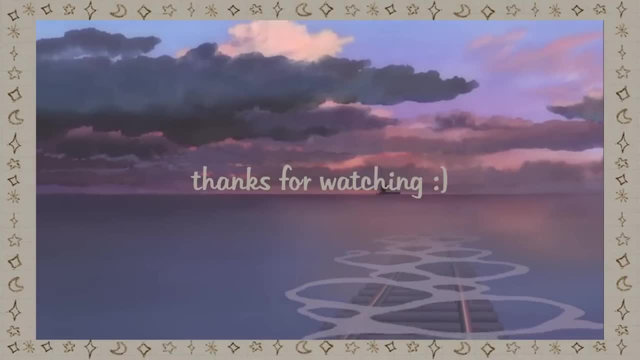 so that's the end of the video. i hope i could inspire you with some of the ideas, because i know whoever you're giving the gift to will definitely love it. so thanks for watching and see you in the next video. 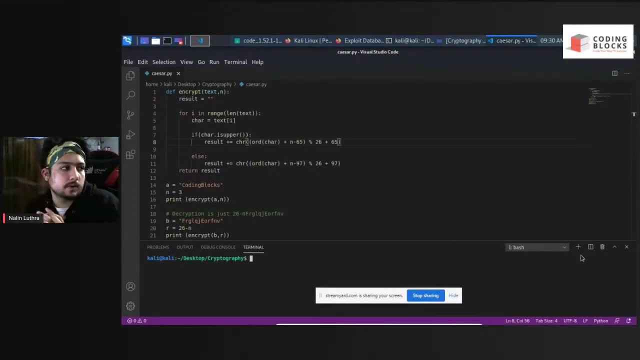 Hey guys, what's up? I'm Nayan Luthra, your robotics mentor, and we are back with CYPTOGRAPHY 2.2.2.2.. Okay, so last time let me just- I don't know. Yeah, so I installed. 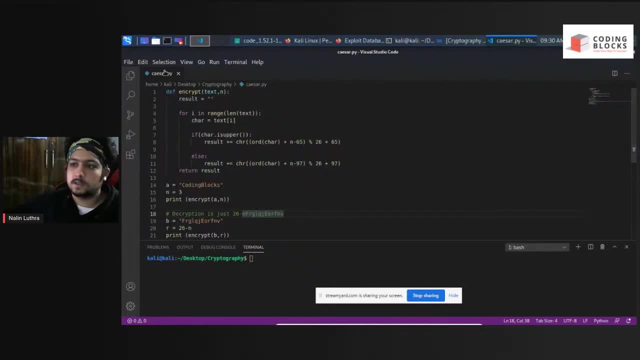 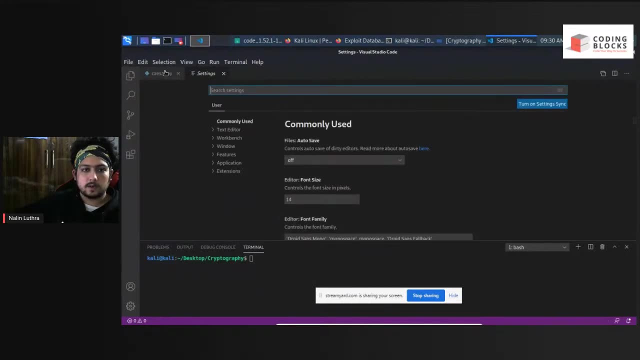 the VS Code because some guys were saying we cannot see it properly in Nano. So I installed the VS Code to itself. You can see the fonts and everything. I can do that for you. I don't know, But it's simple. those who want to do it, you just have to go to where Over here. 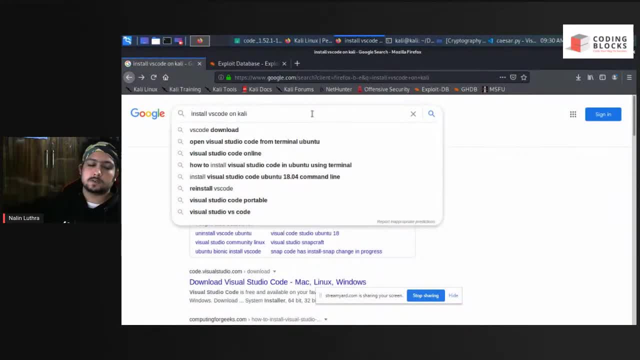 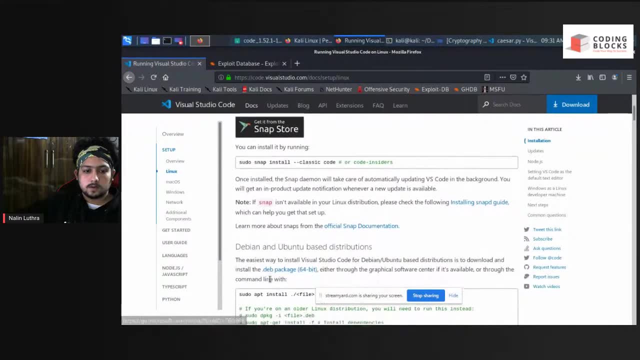 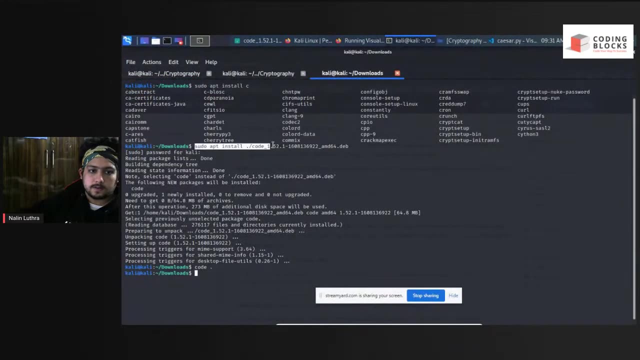 So just go to Google and type: install VS Code on Kali. Click over here. It's good, yeah, And we are good to go, Just write the command. So what the command is? it's quite simple, Just write this: okay, Write sudo app. install whatever Kali. you got right. 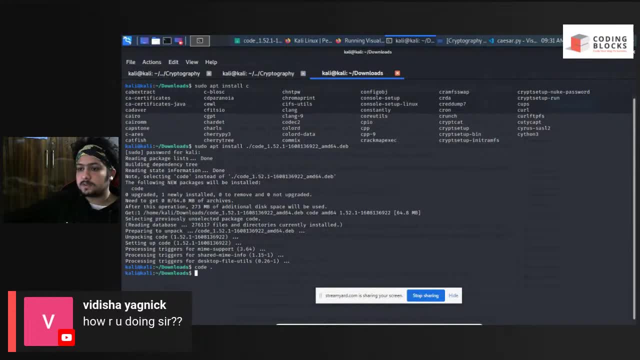 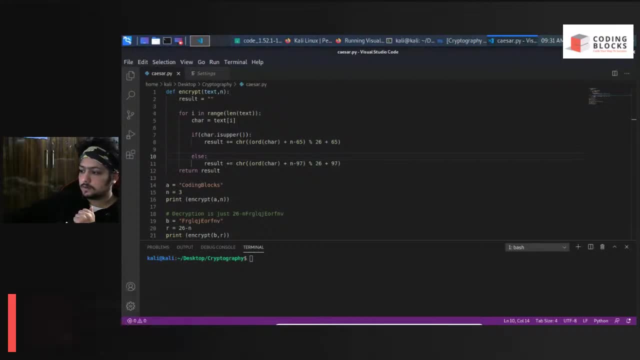 So okay. So I'm just telling you guys that I installed the VS Code from the previous one because many people were complaining that you cannot use Nano properly, So I installed the VS Code, That's all Okay. So it's not important, guys, Let's leave. 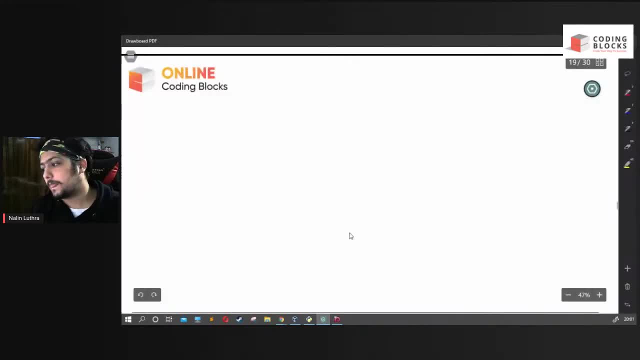 this one for first part, Coming back to itself. So I guess everyone did. saw yesterday's class and worked on Caesar Cipher, right, Okay, All right, Give me a moment, guys. Yeah, So everyone worked with Caesar Cipher, All right?